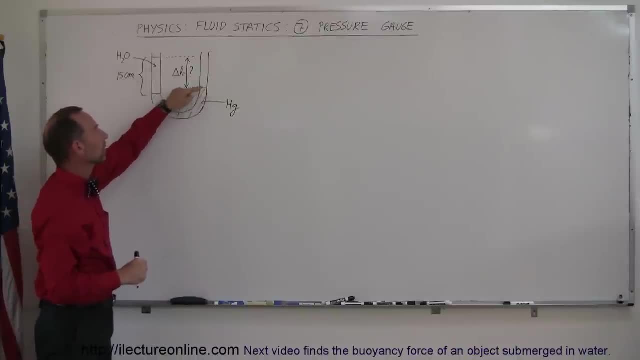 top of the water and it'll push then, of course, the mercury on one side of the tube a little bit higher. and then the question is: what would be the difference in height between the top of the water on one side and the top of the mercury on the other side if the column of water is 15 centimeters? 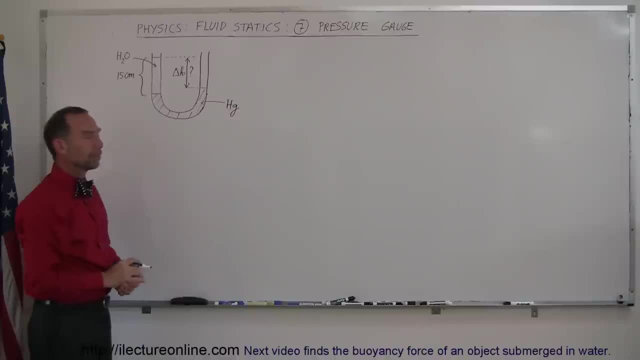 high. So how do you do a problem like that? Well, the best way to do is find the place in the tube, somewhere where you can say that the pressure is the same. and if I take the very top of the mercury on the left side which is being pushed down by the water, and I go straight across the 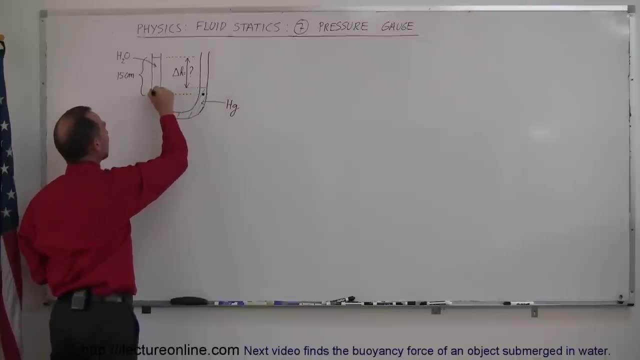 other side of the tube to this location right there, I can say that the pressure at this location must equal to the pressure at that location, because there's nothing wrong with that, But mercury underneath all the way to one side and the other side. so I know that the pressure 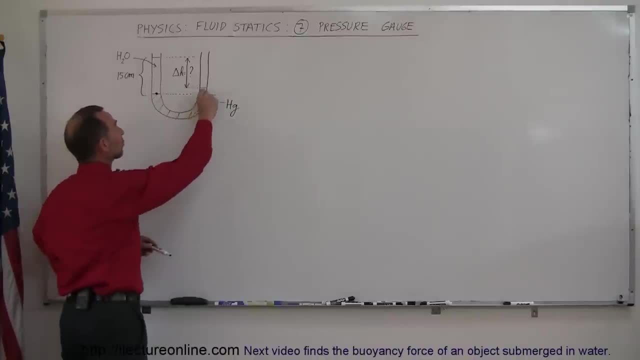 those points are equal, which means that the pressure over here is caused by this height of mercury and the pressure over here is caused by this height of the water. So if I call this pressure 1 at this location and I call this pressure 2 at this location, I can say that 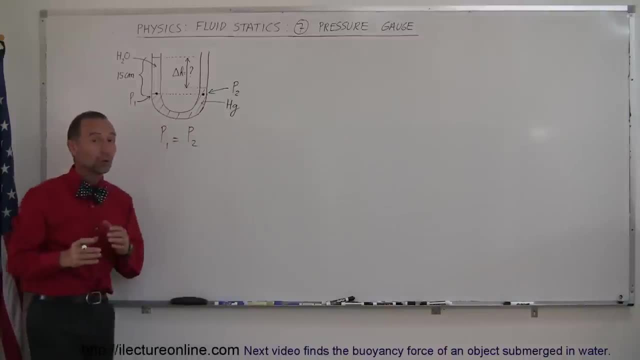 pressure 1 equals pressure 2 and of course we know that pressure inside a fluid is caused by the density of the fluid and the depth of the fluid. So we can say that pressure 1 can be written as rho 1, gh1, which means the density of fluid on this side. 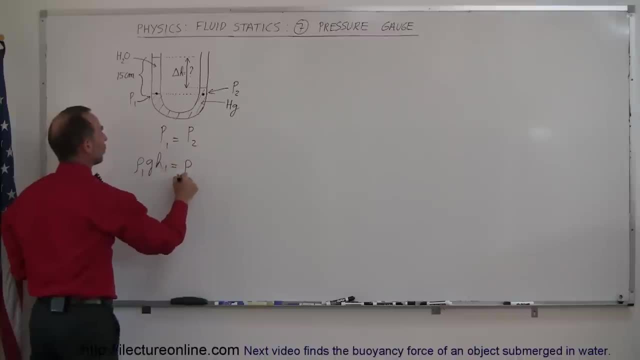 and the height of the fluid on this side equals the rho 2 gh2, which means the density of the liquid above this point on the right side and the height on the right side. So this right here could be considered h2 and this then would be considered h1.. 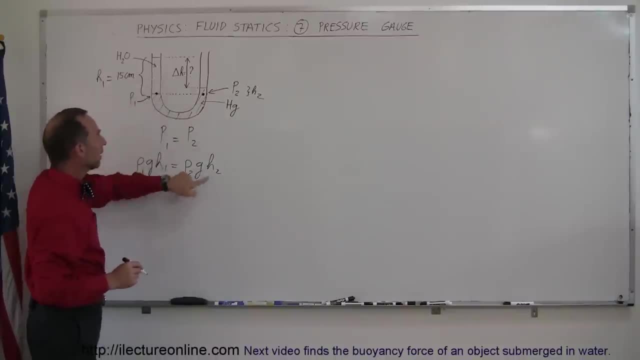 And then density 1 represents the density of water and density 2 represents the density of mercury. All right, so I see a g on both sides, which means I can get rid of the g on both sides, cancel those out, and since I already know what h1 is, I'm going to figure out what h2 is equal to and turning the 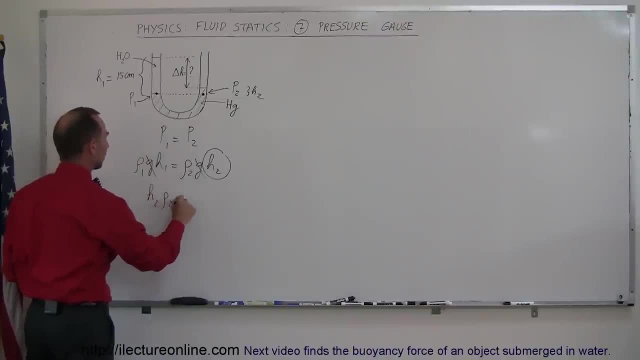 equation around. I can say that h2 times rho 2 is equal to h1 times rho 1, and then, dividing both sides by rho 2, I can say that h2, which is the height of the mercury above this point, is equal to h1 times the ratio of rho 1 divided by rho 2..